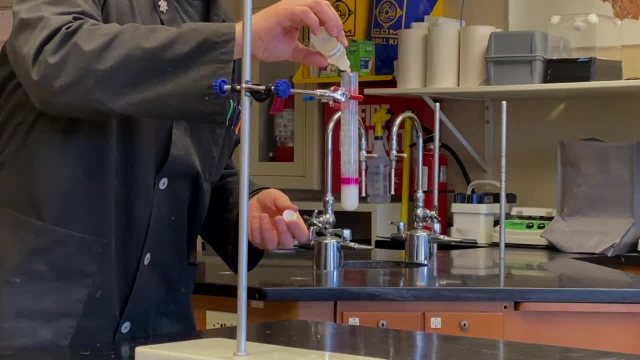 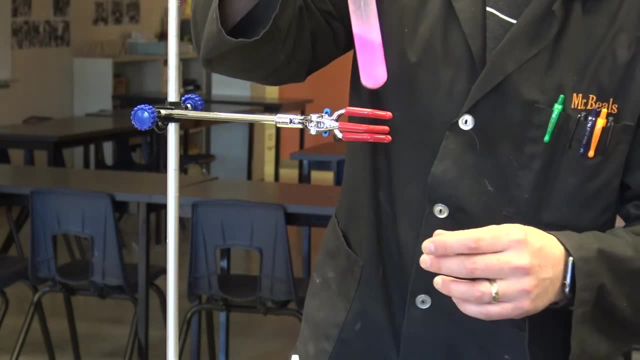 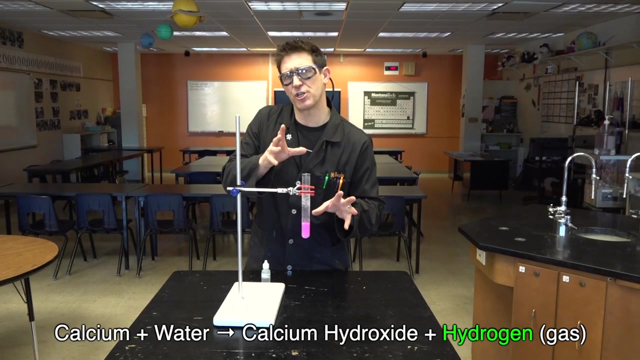 why I like to do this at Valentine's day? because, well, okay, all the colors, of course, are Valentine's-y. So this is a very basic solution. the opposite of acidic. So this is nice, but if we're producing hydrogen gas, that hydrogen gas should be flammable. Let's look at this again. 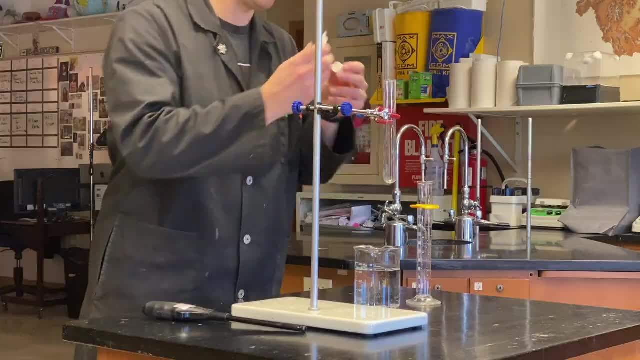 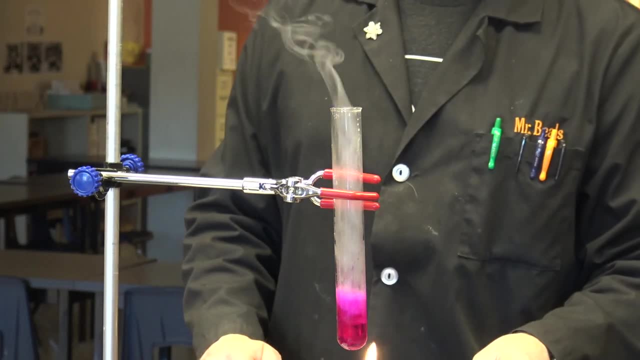 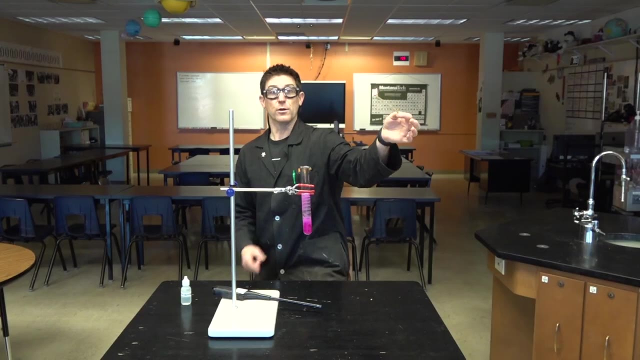 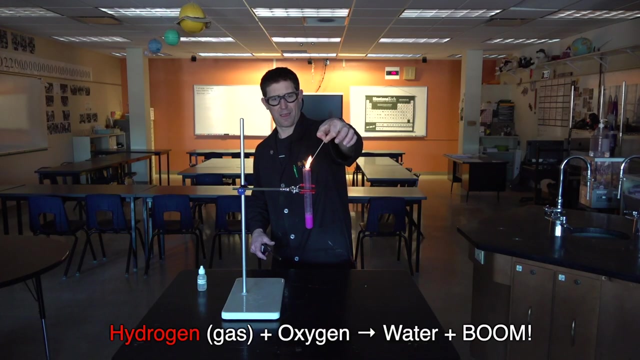 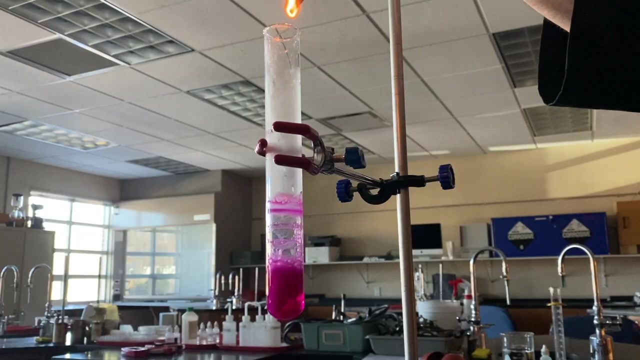 This time I'll add the phenolphthalein indicator ahead of time. So here goes nothing. Oh, yeah, Ready. Oh, did you see it? Oh, let's turn the lights off. Oh, you see it. Oh, if this is fire and ice experiment, well, there's our fire. Where's our ice? 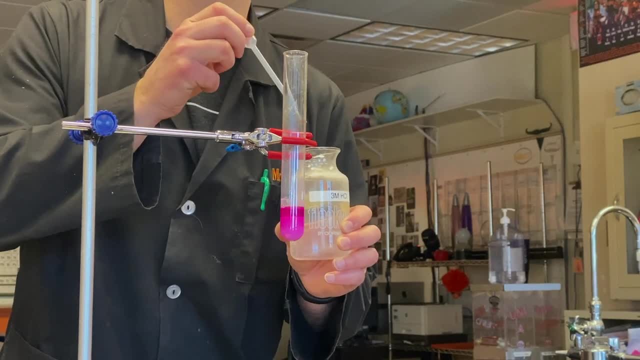 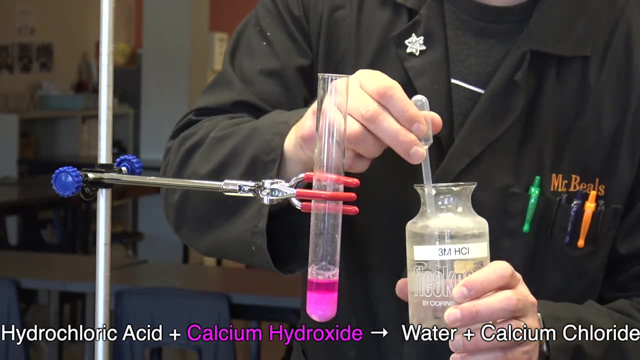 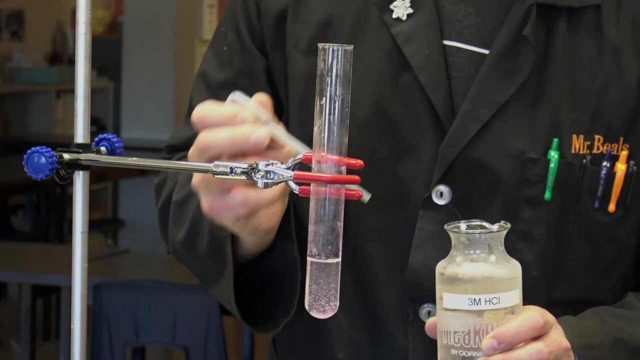 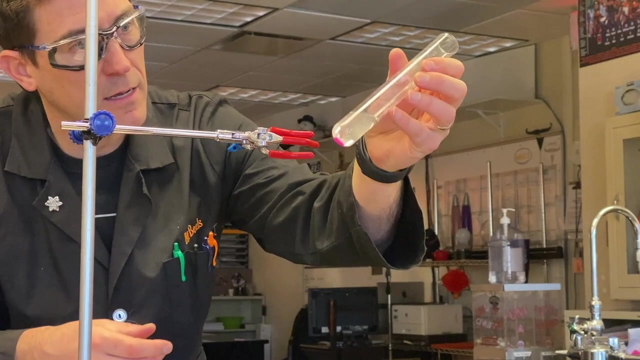 I'm going to use some hydrochloric acid. So we're going to get a reaction now where the acid from this is going to react with the base, the calcium hydroxide in here. Let's see. Whoa wait what Look? the whole thing we just made is gone. 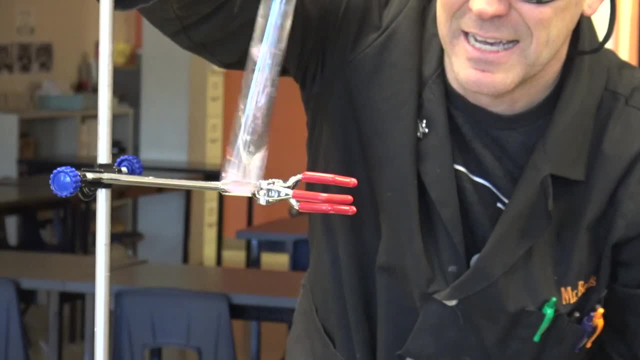 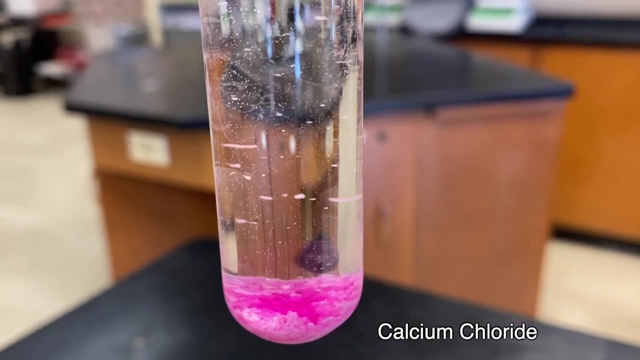 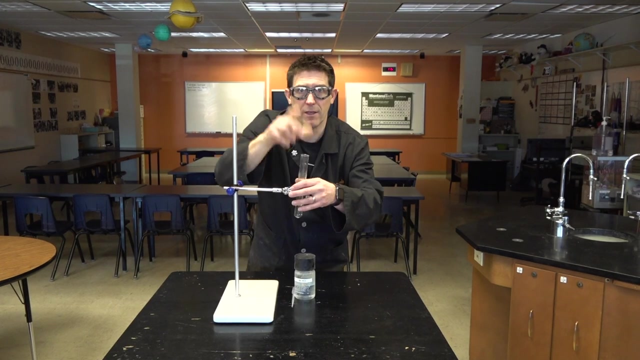 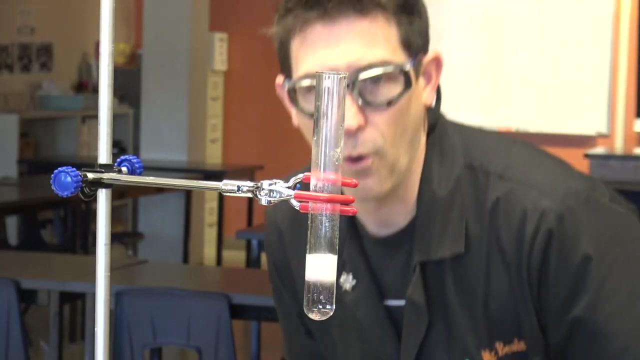 Except for some little teeny, tiny pink snow crystals in the bottom. We've made our little snow globe here by a whole series of reactions. Now we can, we can- make this thing good. Should we keep it going? Produce more hydrogen gas? Huh, Oh, oh, wait a minute, Wait just a moment. Can you see that? 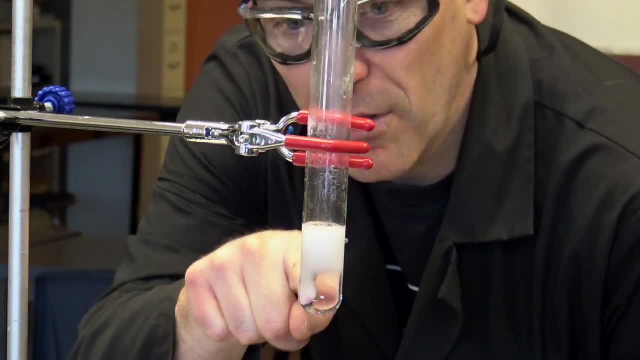 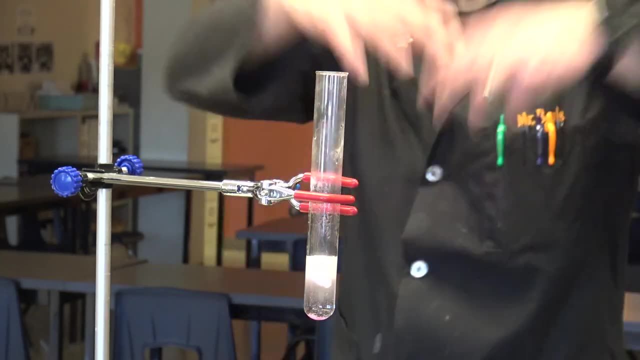 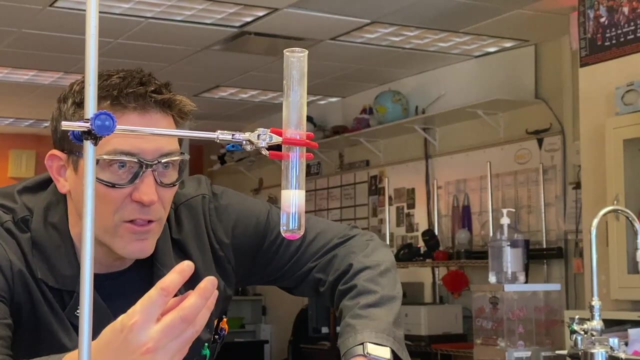 Can you see the snow falling in? Oh, There we go. We've got so many things going on And now it's starting to turn pink again. We're getting snow crystals that are falling down. Look at this. Should we add some fire?